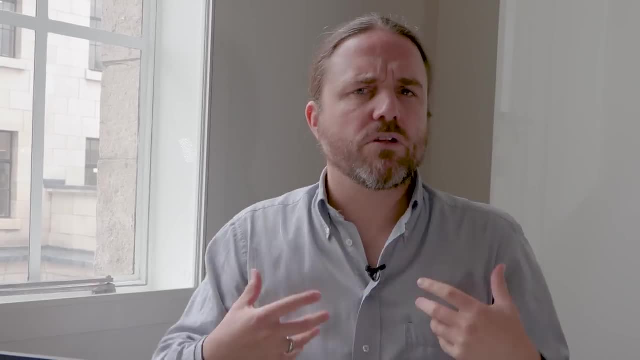 And what they do is they give us a language that much more readable and much more writeable and much more intuitive. And so what they do is they give us a language that is much more readable and much more readable and much more writeable and much more intuitive. And what they do is they give us 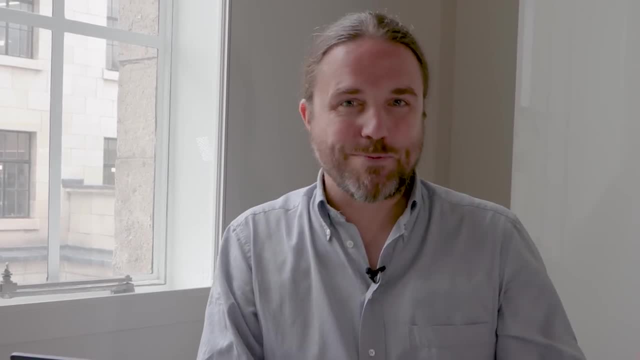 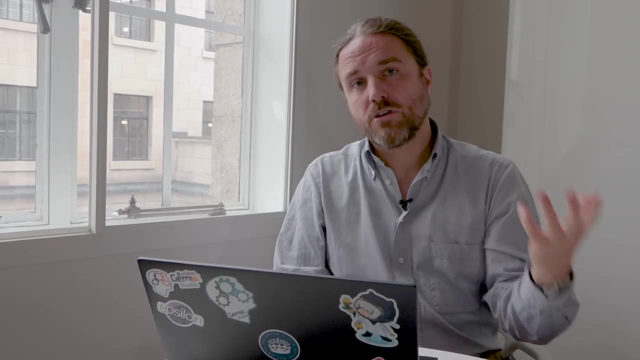 a language that is much more understandable to a well-trained human being. There's still a problem with that, okay, Which is you've got to be a technically trained person to use these languages, because what these languages are doing is they're allowing you to express a problem and a solution. 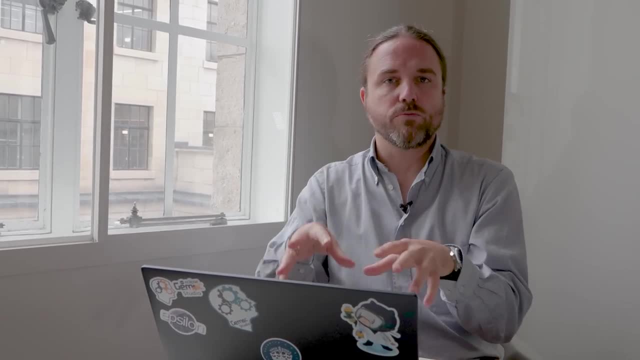 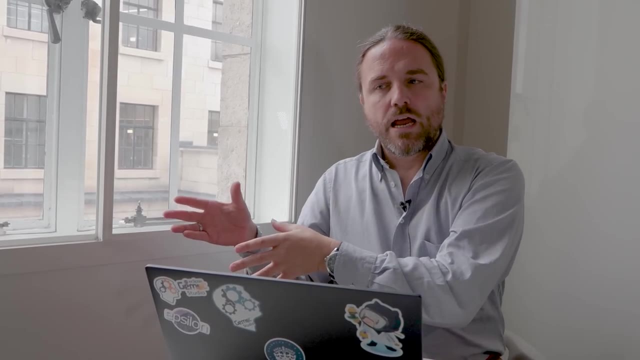 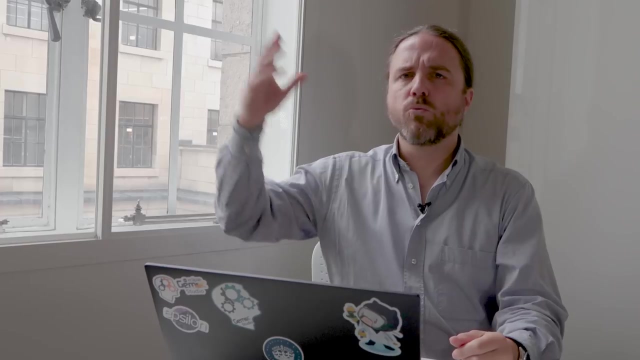 to the problem that you have in terms of a computer. So you've got to say: computer, do this computer, do that, now do this. But actually the problem that you had was: I want to manage bank accounts, I want to manage mortgages, I want to simulate cell biology. 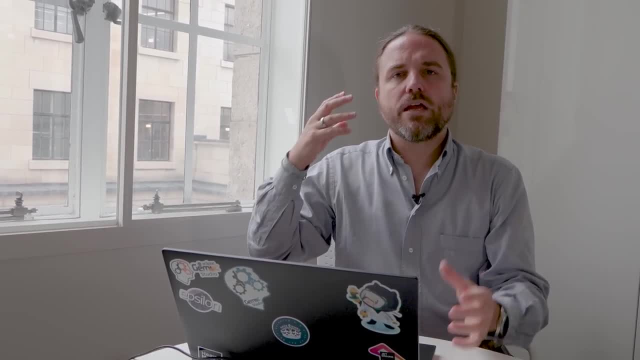 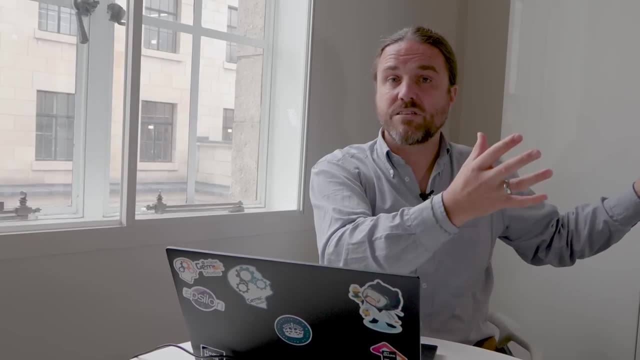 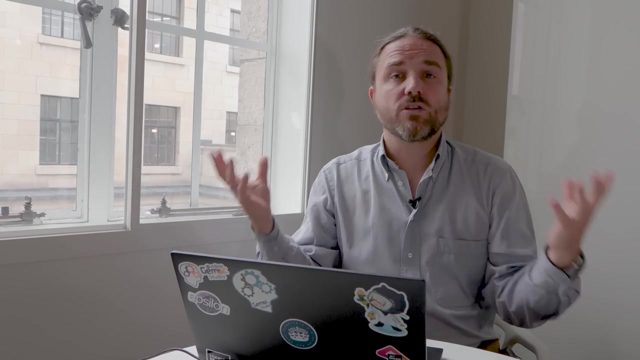 Problems that the computer doesn't have a clue about, basically. So in the programmer's head there needs to happen a lot of translation from these domain-specific concepts into something that explains them to the computer, And all of that translation. and all of that translation gets lost. Maybe let me try and show that to you a little bit in a simple 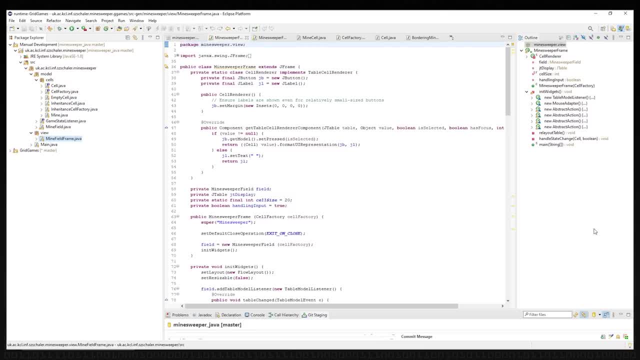 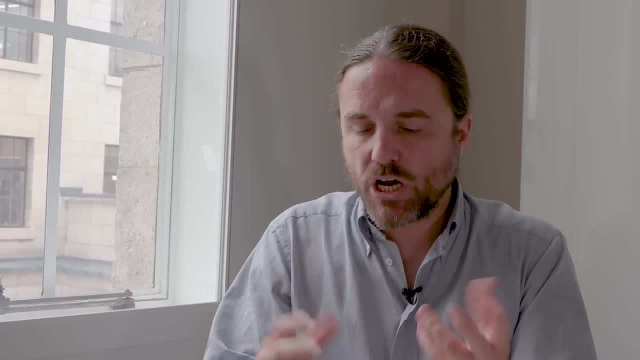 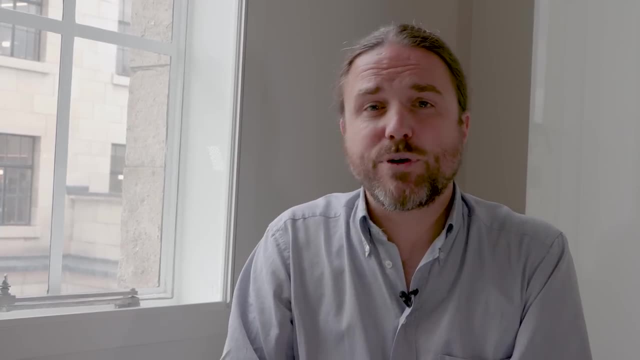 example. What I have here is a simple development environment as many software developers will use in their sort of day-to-day work, And I've written a simple program in Java that allows me to play Minesweeper games. Now, depending on your age, you may or may not know what Minesweeper is, So 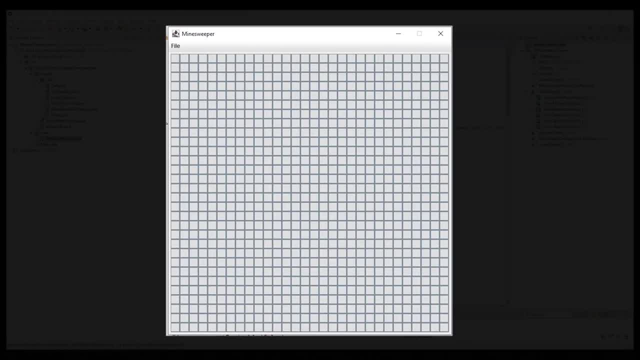 I've brought it up here as an example. It was this sort of game, I think it was- came with pretty much all the old computers. It was a lot of the old computers but it's got a lot of the old hardware. 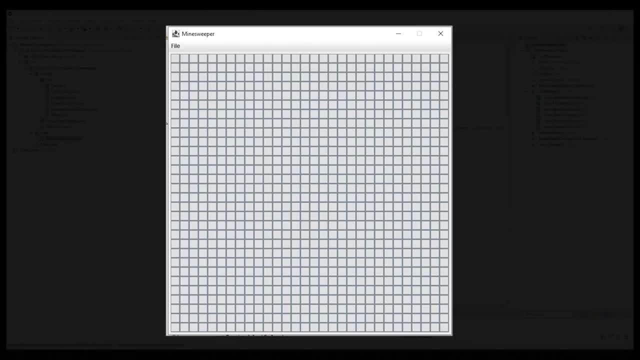 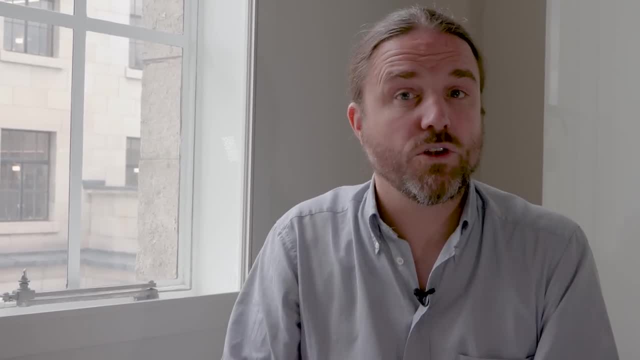 computers and where you've got this sort of rectangular grid here, and each element on the grid potentially hides a mine, and your goal is to find all the mines without stepping on one and exploding them. and so the way you do this is you click on one of these cells and it then tells you: 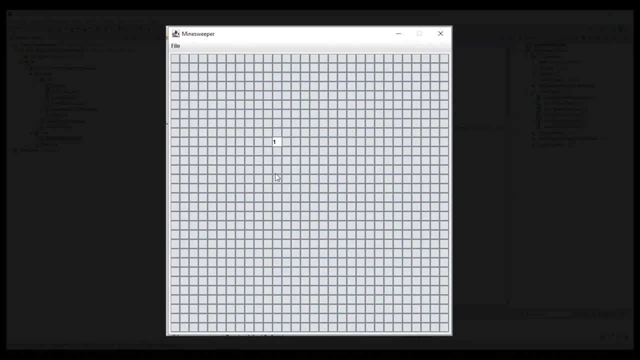 whether there is a mine there or not. and if there wasn't a mine, then all is fine. and, as in this example, here you might see a little number that tells you how many mines are in any adjacent cells. now, in this case that doesn't help me much, because it tells me there's one mine, but but you know not. 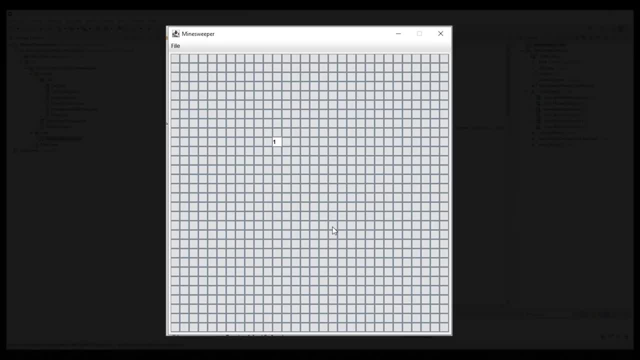 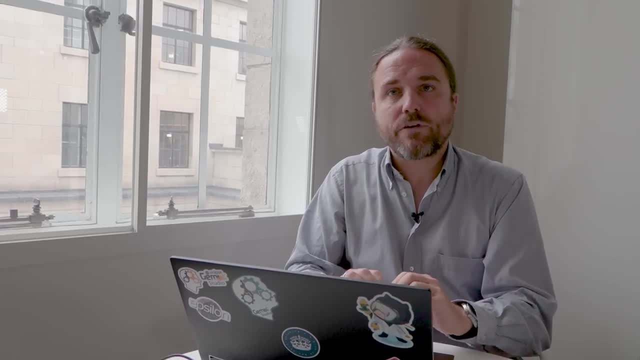 a lot else. so let me click somewhere else to get a get a bit of a start on this. and you see, oh, this was better- i've clicked on an empty uh cell here where there's no mine. i was got lucky, um, but i got so lucky that i actually found that there's lots of empty cells everywhere around and it'll. 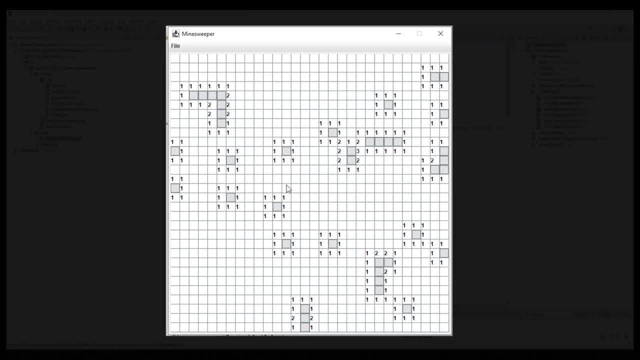 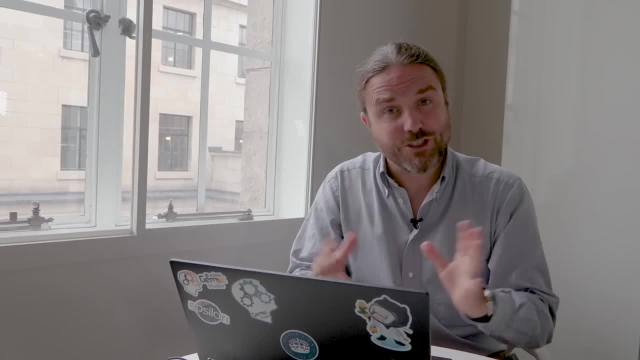 automatically open all of those up and how i can go and i can work out with these numbers where the mines are. now the goal of this video isn't to explain minesweeper to you, so i'm going to kind of stop at this point, as much as i love playing minesweeper- minesweeper, and i'm going to look. 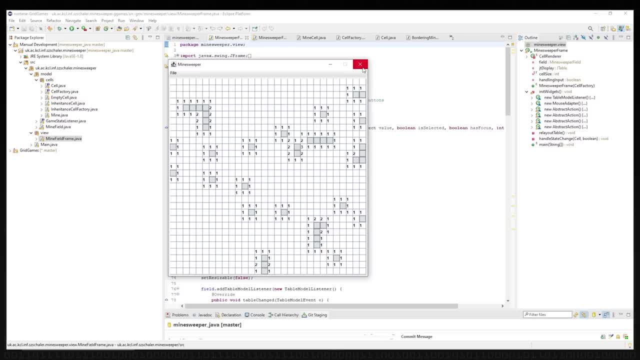 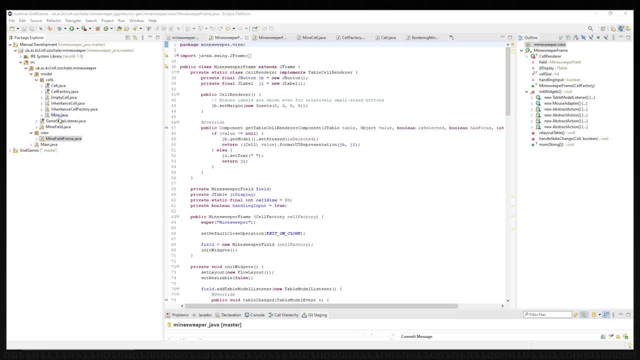 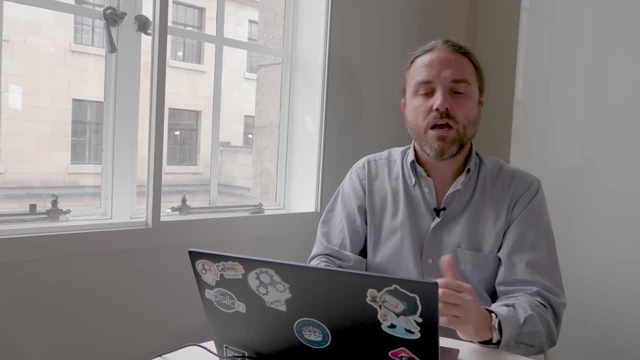 pieces, all the various files that I've built to build this program. Now, Minesweeper is, by no stretch of the imagination, a complicated piece of software. right, It's still a fairly simple piece of software but you can still see. you know, as I developed this I sort of had to write. 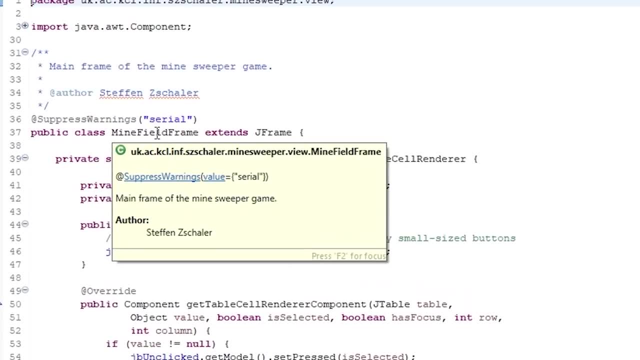 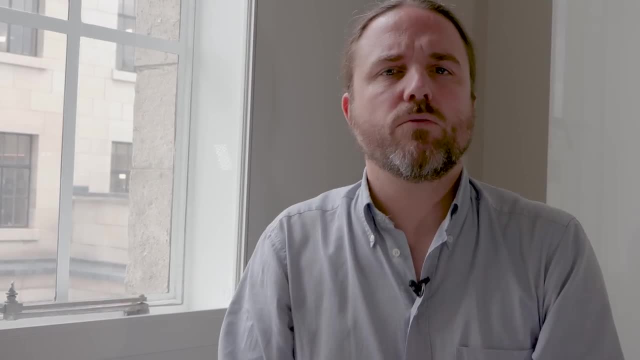 quite a number of files, Okay, And if I look into some of these files, this is one of the classes. it happens to be the one where everything starts And you can see there's a lot of code going on. Now, a key question you might wonder about with Minesweeper is: what are the rules of Minesweeper? 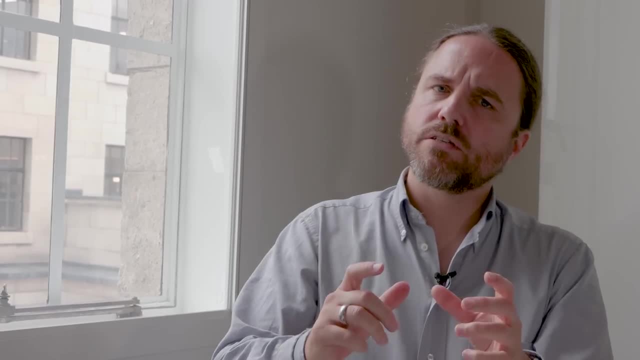 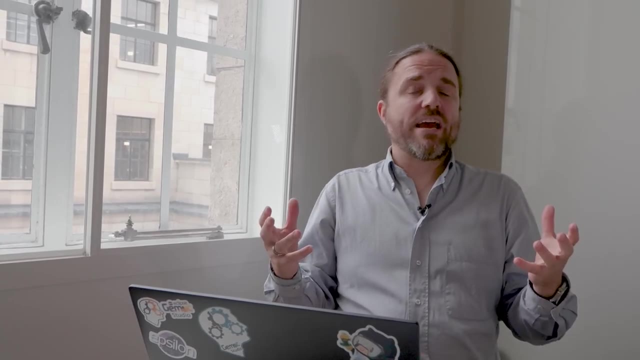 and how do I change them right. If I want to build a slightly different version of Minesweeper or slightly different rules, how do I do this right? Because that's, in the end, what you care about As a game developer. you care about the rules of the game. You don't necessarily care. 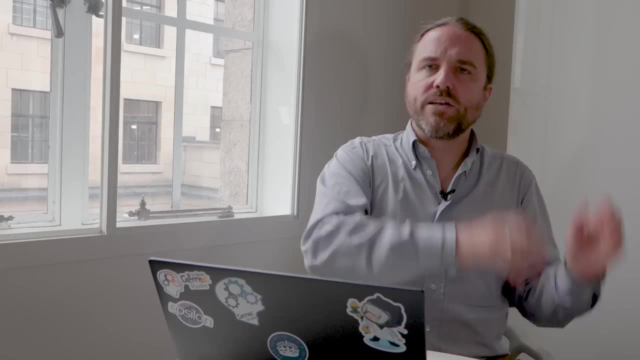 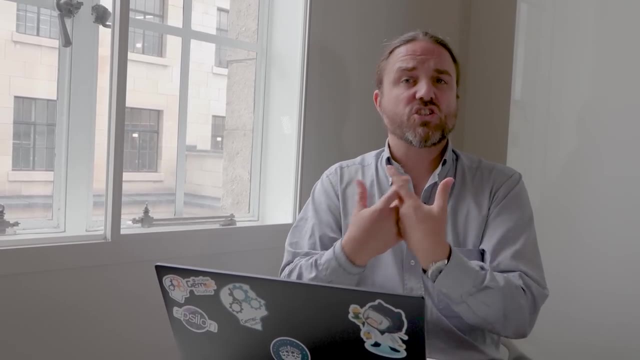 so much about how to explain to Windows or Linux Or Mac OS or Android how to get the thing on the screen. In the first instance, you're interested in designing the rules of the game and you want to be able to see them, and you want to be able to. 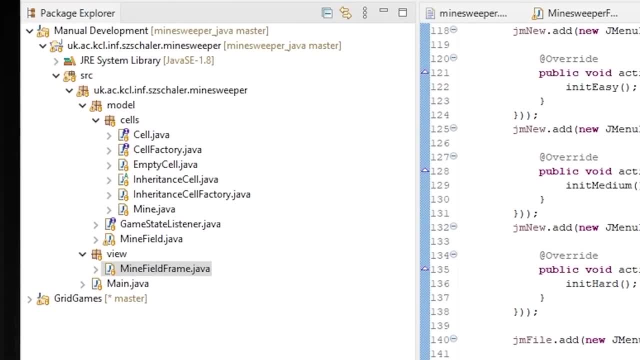 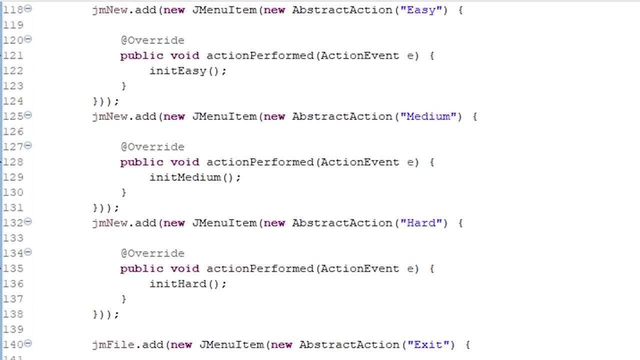 change them. The problem with this code, of course, is we've got nine classes or so here and the rules could be anywhere in there. Okay, In fact, there's all kinds of other stuff in this code, right? So this code here that we see here, it's got stuff about the menu, It's got stuff about initializing. 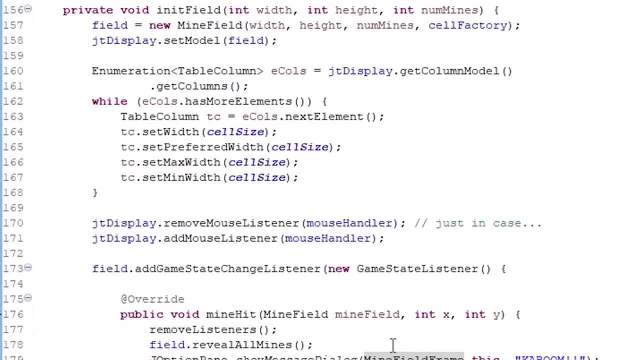 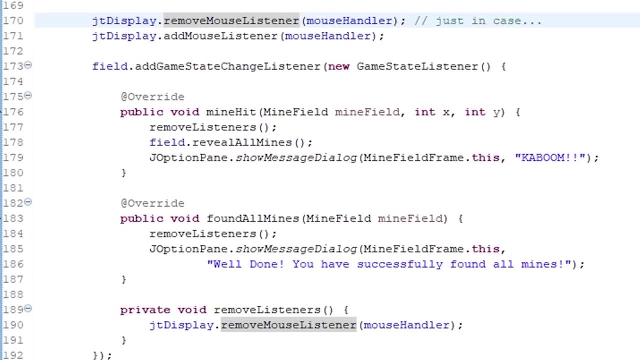 fields. But then in there, if I look at this again, it creates tables and it creates listeners to mouse. again, That's about user interaction and not so much about the rules. It's all kinds of things are intermixed right And it's really difficult to find what the rules of the game are. Okay, In an 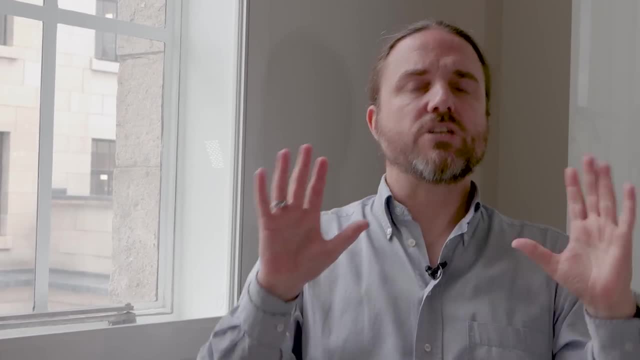 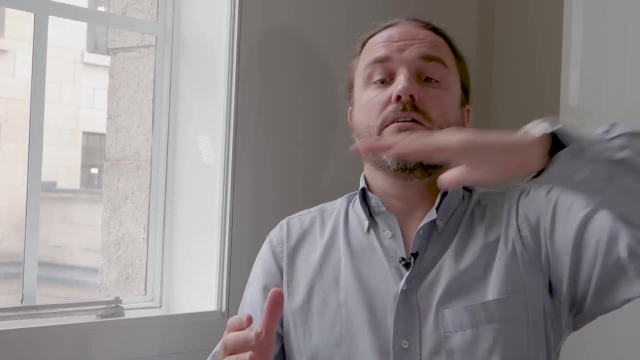 MDE approach. what we would take is we would take a step back from this and we'd say, actually, let's not worry about all of these details, Let's abstract away from them, just like Java abstracts away from the machine code. Let's abstract away from that and build ourselves a. 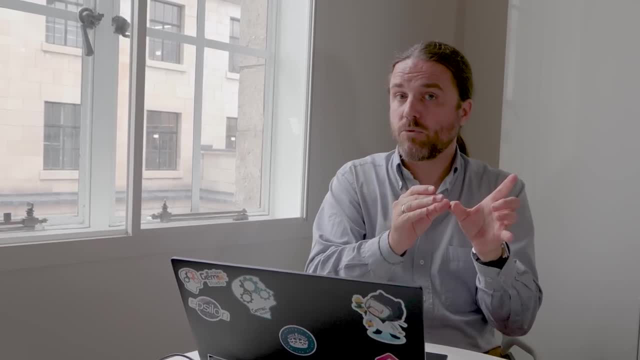 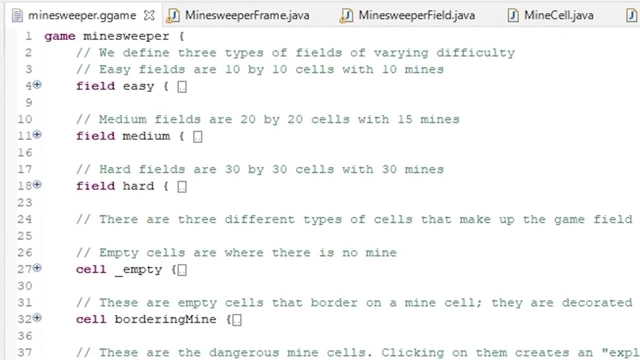 modeling language and then write a model that captures only the information that we care about. Okay, So let's look here at a different way of representing Minesweeper in this file here. So this is a little modeling language I built and a little model in that modeling language I built. 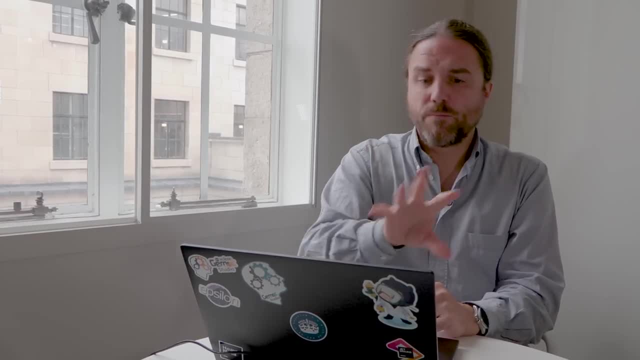 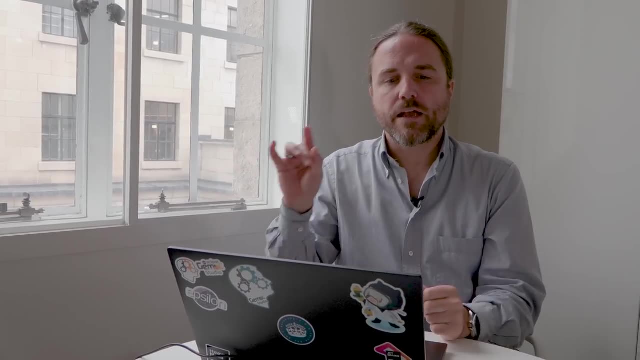 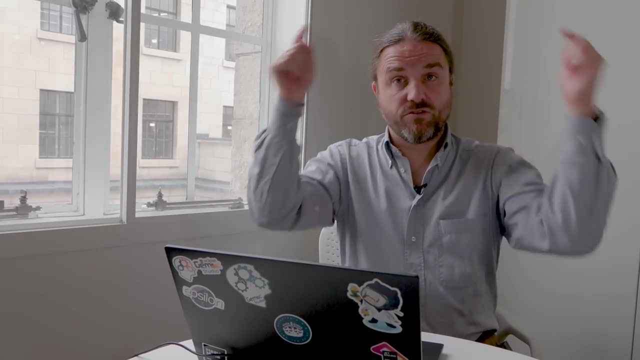 to describe Minesweeper, And in fact, it turns out that from this model, I can generate automatically all the Java code that's needed for running Minesweeper. Okay, And what this does is it has these field commands here which allow me to define what fields there are, what the rectangular fields, 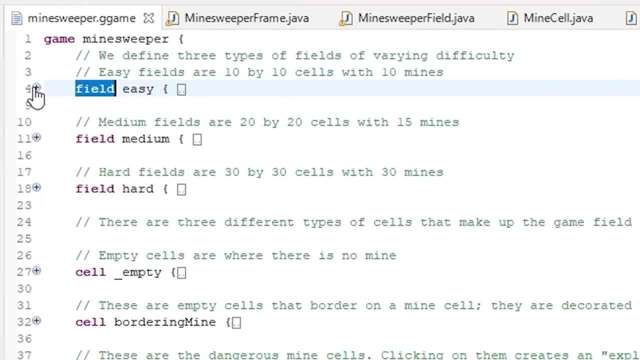 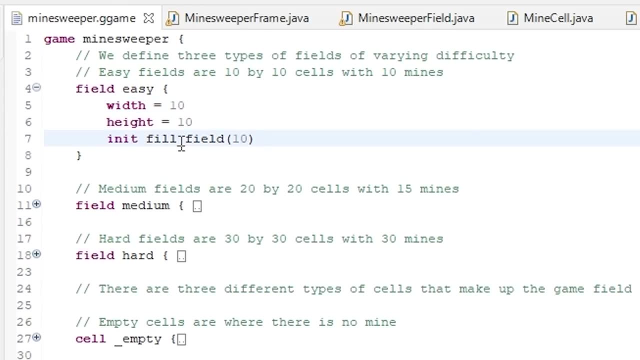 Let's open up one of those. So the easy field here. it basically says, well, it's 10 cells wide, it's 10 cells high, And then it's initialized using this fill field thing which is defined down here, And it has takes one parameter, which is the number of mines that we want to set up in. 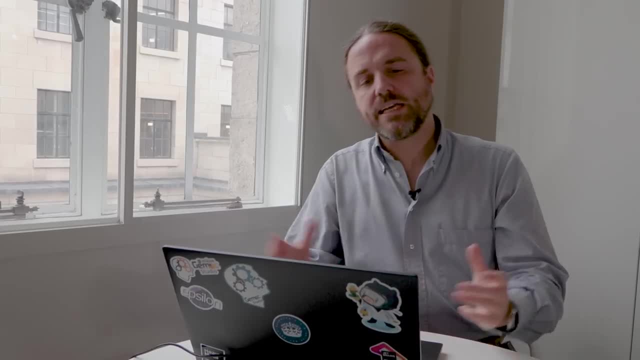 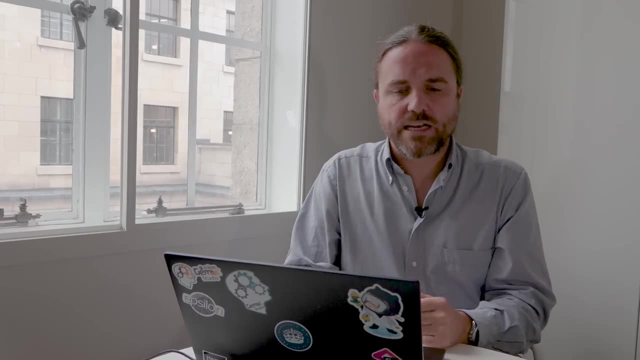 our field And we're setting this to 10.. So in an easy field we have: it's 10 wide, it's 10 high and it contains 10 mines. Okay, Now the other fields are set up with different sizes, et cetera. 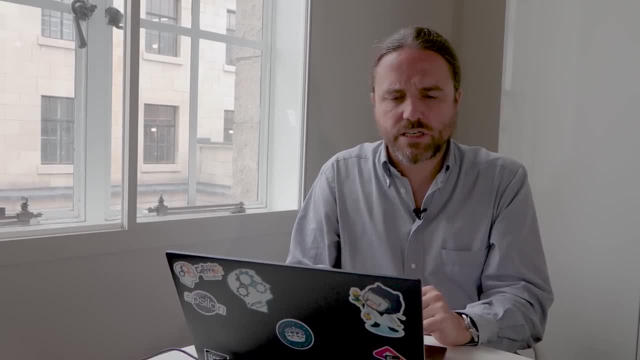 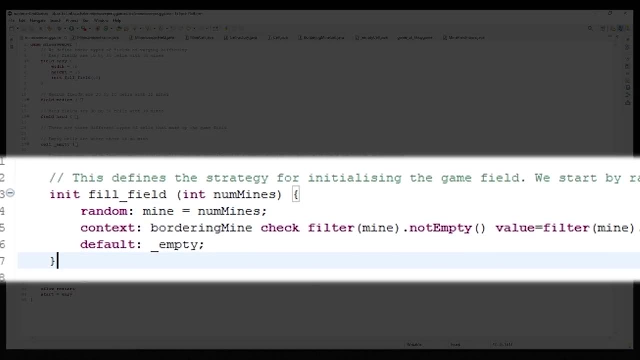 Let's have a look at briefly at what this fill field thing looks like. Well, it sort of says: okay, I'm going to use various strategies for initializing the field. I'm going to start by randomly initializing this many element cells in this field with mines. Then I'm going to use 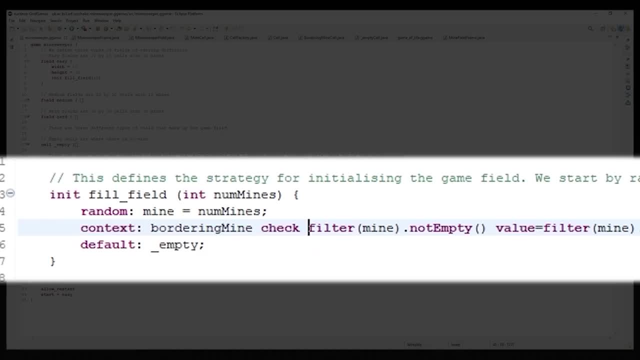 this context rule to say: I'm going to put bordering mine cells anywhere where there is already a mine cell somewhere And they're going to sit around that And the bordering mine cells are the ones that show these little lines, And then I'm going to put a bordering mine cell. 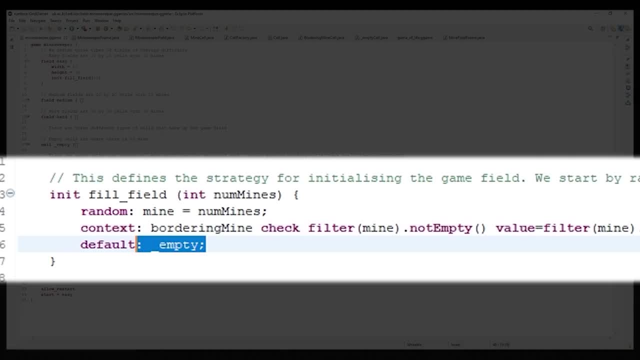 anywhere where there is already a mine cell somewhere And they're going to sit around that And then everything else gets filled with empty cells. Okay, And that's the basic things that you need to know about setting up a minesweeper field, right? So you don't need to know more, You don't? 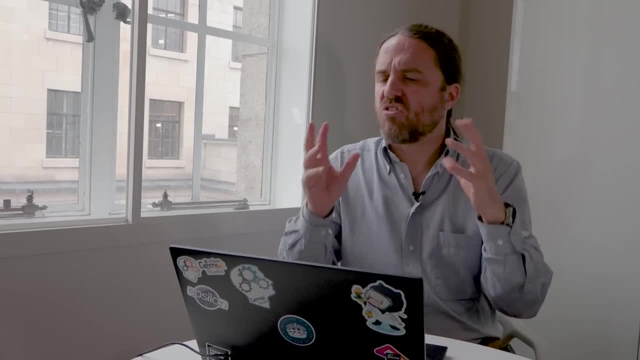 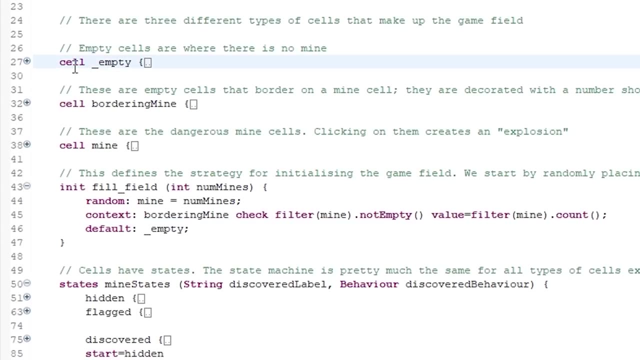 need to care about how this setting up of these cells actually happens, or anything like that. You just want to say that's the rules, Okay, So we've mentioned these different types of cells, So obviously we need to define them and that's what the cell command is for, right, So we can. 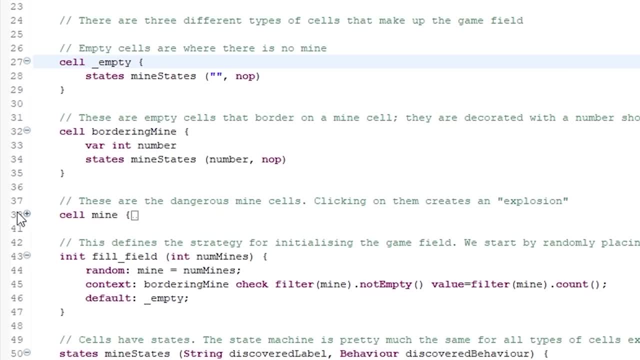 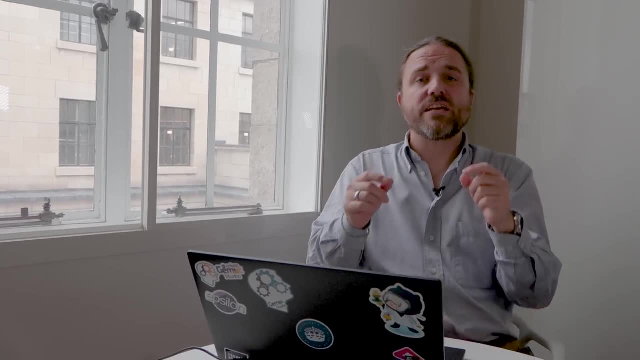 define an empty cell, We can define a bordering mine cell and we can define a regular mine cell, basically all set up using these mine states thing here. because the key idea in this modeling language is to say: well, actually each of these little cells that we have here has a little state machine attached to it. 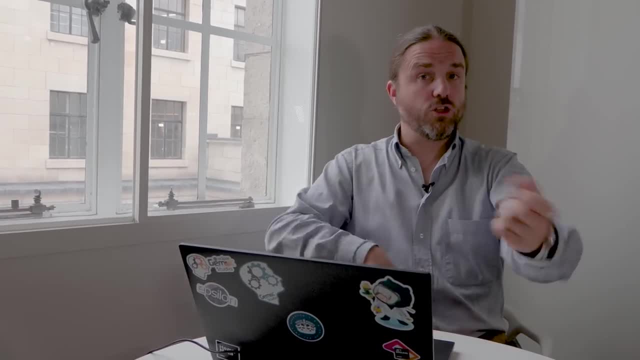 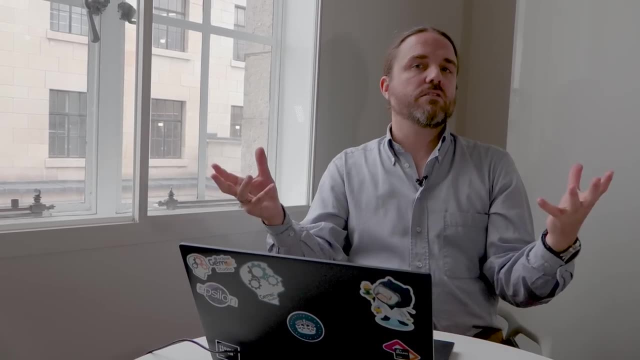 Okay, So it can be in one of a number of states and, depending on what the user does with the cell and depending on, maybe, what else happens, it might change its state. Okay, And so it's useful to just basically be able to do. the rules of the game, I guess, are what states there are and what the 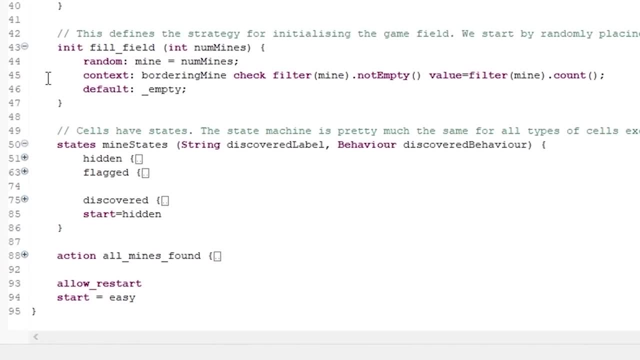 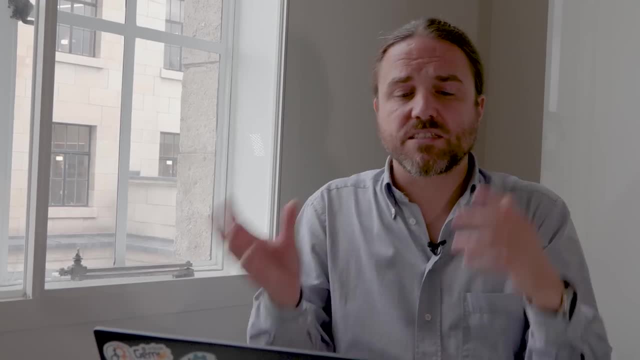 transitions between those states are, And so we define what the state machine is here using this mine states thing here, And you can see that pretty much the state machine is the same for empty cells, mine cells, bordering mine cells, because essentially they react to user input in. 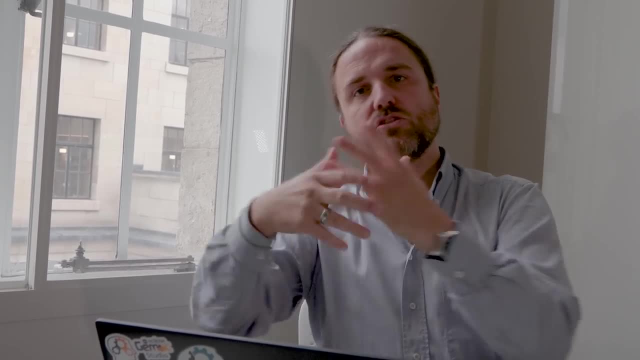 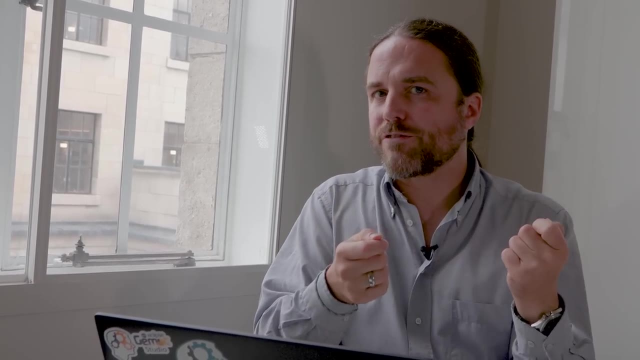 the same way. They go from this undiscovered state, this hidden state, to a discovered state, and maybe you can add a flagged state if you wanted to. The only difference is that they might be showing slightly different things on when they're discovered and there might be a. 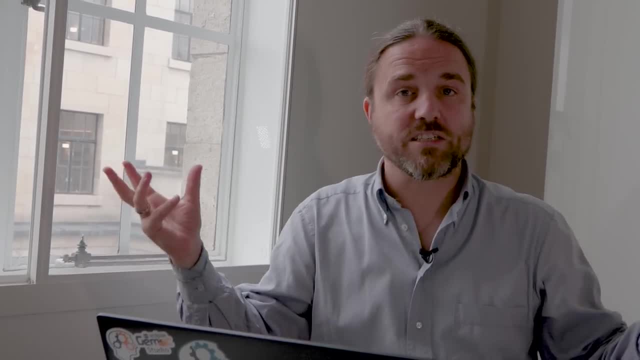 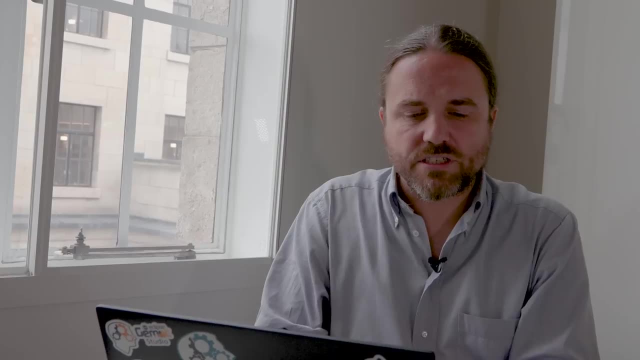 different thing that happens right When you click on the mine, things will explode. When you click- not don't click- on the mine, nothing will explode. So you can see that the state machine is. the same thing will happen, other than discovering the cell. And then we say, okay, well, what are the? 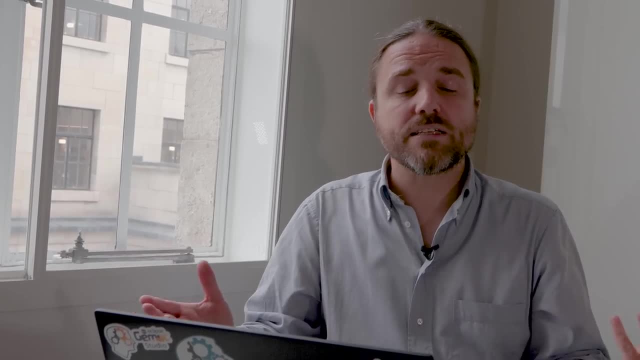 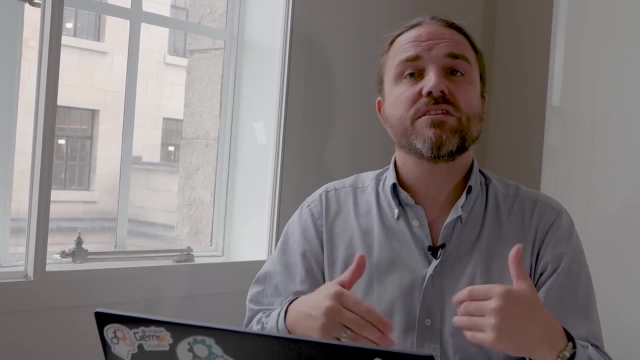 states? Well, it starts with this hidden state, And what's important about the state? Well, what's important is what it looks like. It looks like a button with no text on it, like an empty button, And what happens when you click on it or when other things happen? right, So transitions that. 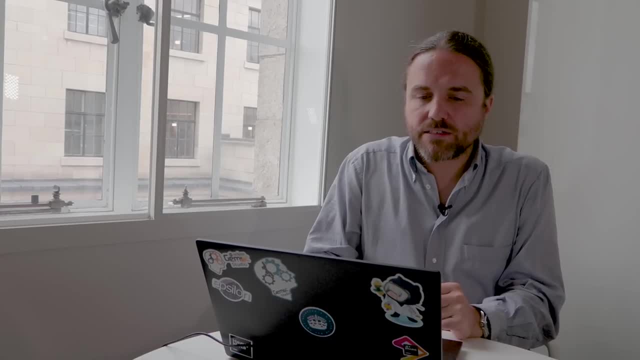 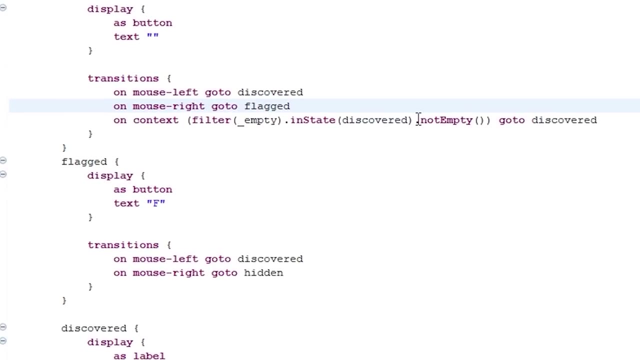 move it to another state. But now we can do things here right Quite easily. we can say: oh actually, let's not go to the flagged state when you right click on the cell. Forbid that, Let's not introduce this flagged state. right, The flagged state is where you can. 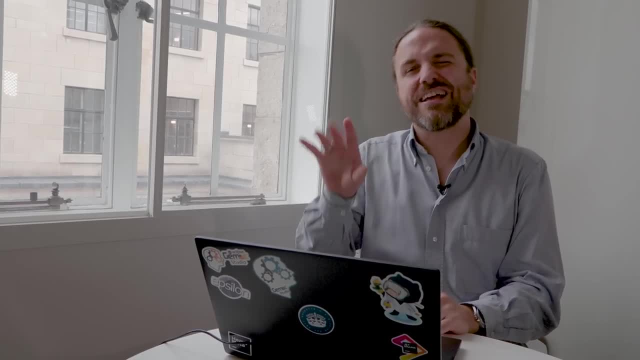 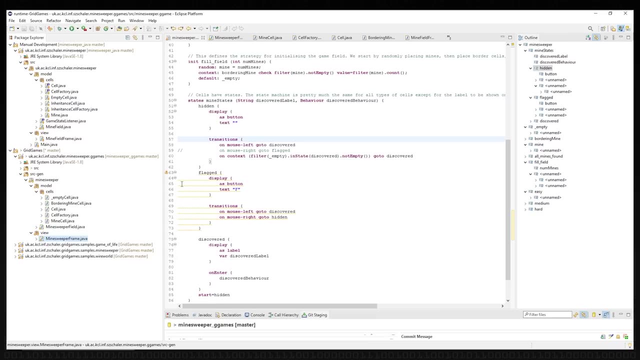 right click on a cell and you can sort of put a little marker there, to kind of go. I think there might be a mine here, but I'm not quite sure. And if I save this here, then it regenerates code for me. Now let me just run this And there we are. There is my minesweeper, And now I can try and 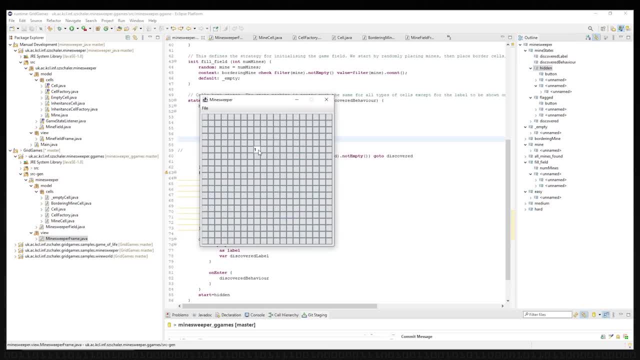 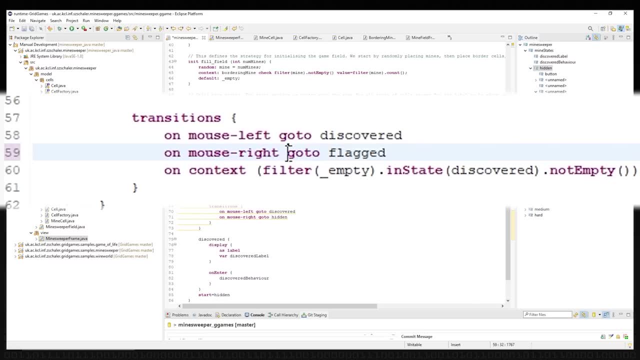 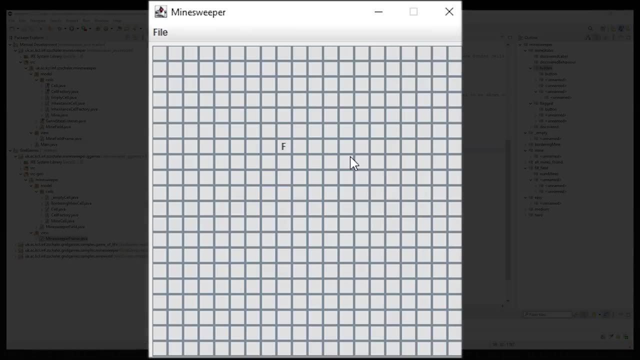 right click on these, but nothing's going to happen. But I can continue to sort of left click and play the game. Okay, This thing, available again here, regenerates all of this code for me and I can run it again. And now I should be able to right click on here, See, and I've got the flagged this cell here to. 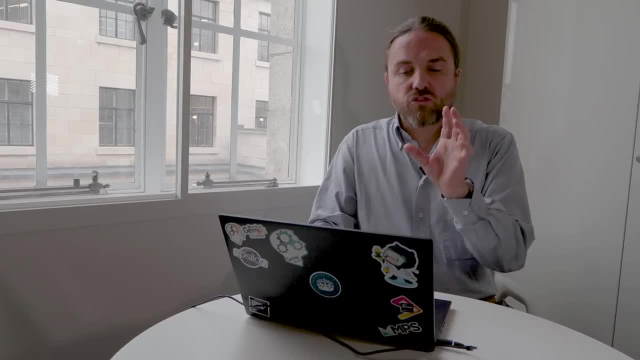 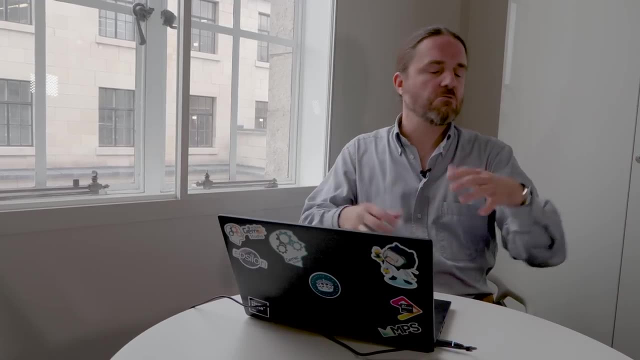 say there might be a mine there. I'm not quite sure. Okay, So really easily, I've just changed the rules directly in this. Imagine if I had had to try and do that in my Java code, I would have probably had to touch three or four files. remember the changes that I made. make sure that I make. 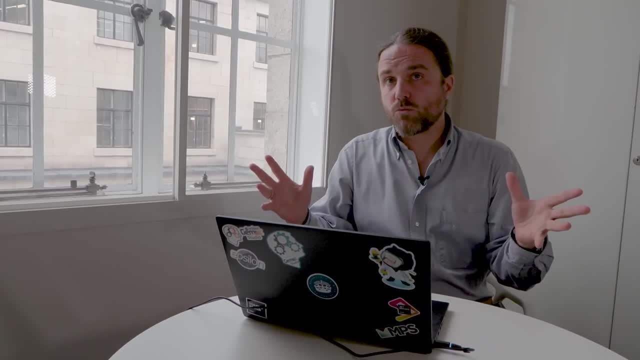 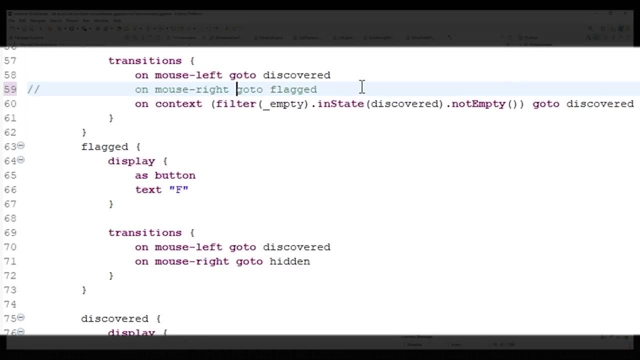 them consistently, et cetera, none of which I had to worry about in this case. Okay, Another thing. you might have spotted that briefly. if I comment this out again for a moment here, you will see. suddenly this part of my model gets this yellow underline. I go on this. this says this state: 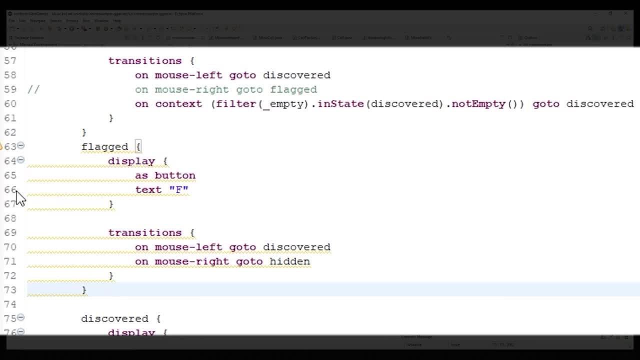 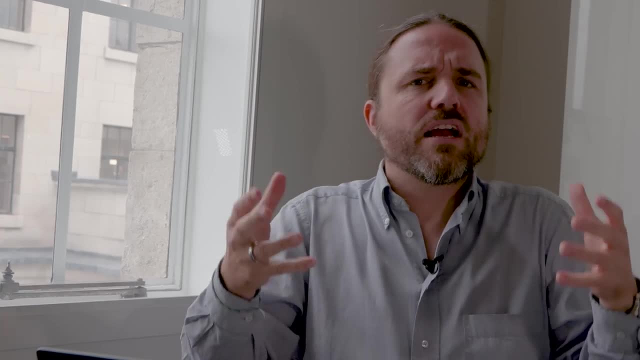 cannot be reached. So this is only possible because in my model, I have made it explicit that there's this idea of a state and that there's this idea of things moving between states, And therefore, clearly it's not a good thing if I've defined a state that cannot be reached. 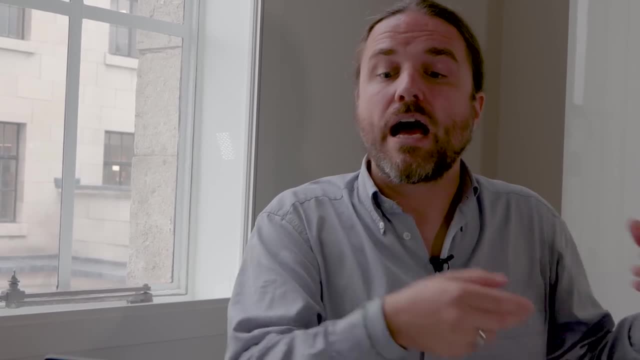 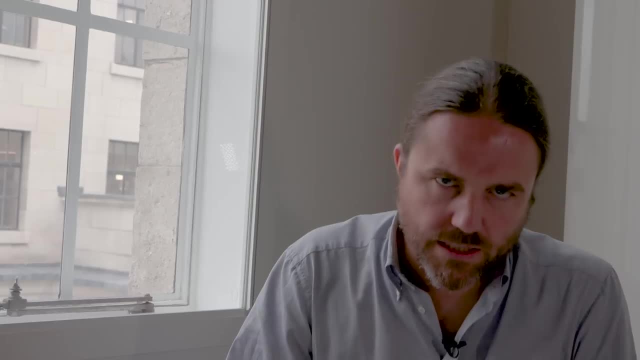 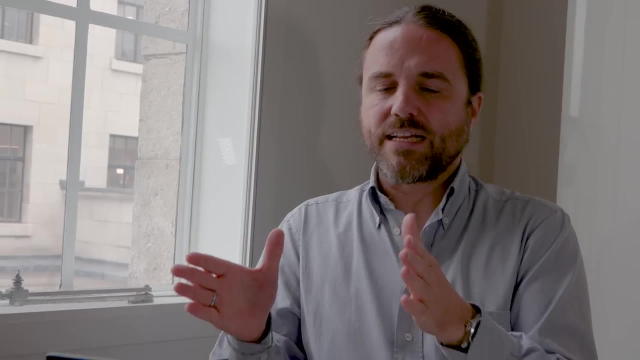 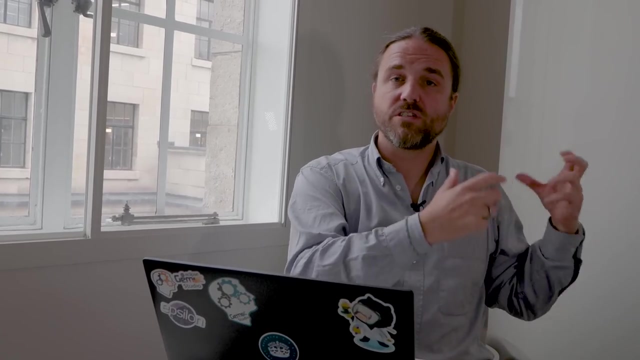 this was a language that only allowed me to build Minesweeper. it'd be a bit silly, Okay. So the trick to do in MDE is to build languages that meet, find that sort of sweet spot between being specific enough that the abstractions are useful to a particular group of people and that they 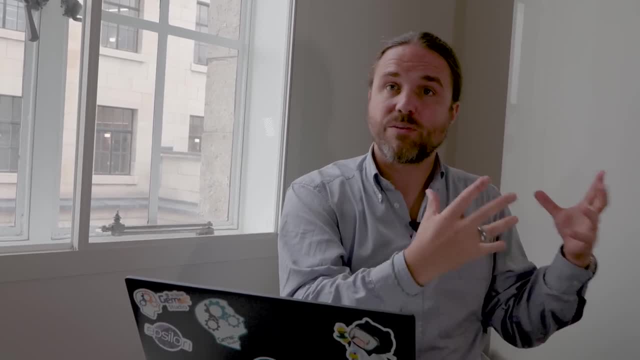 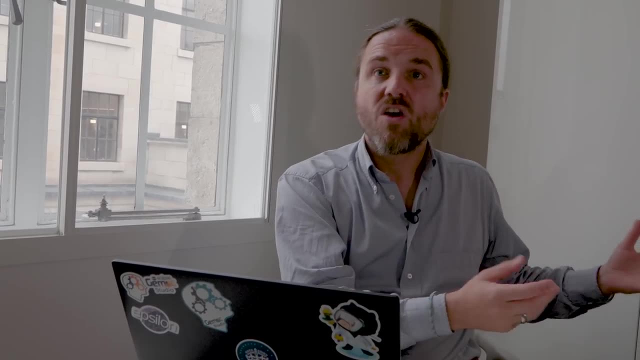 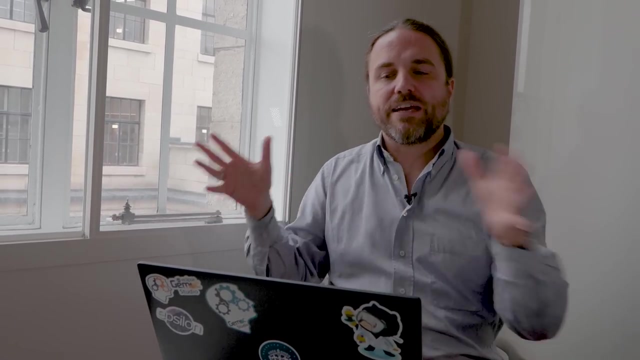 allow us to do, give compact expressions of the things that we actually care about, And allow us to do useful analysis and validations like the one that I've just shown, While not being so specific and narrow that we can only write- ever write- one program in the language Okay And 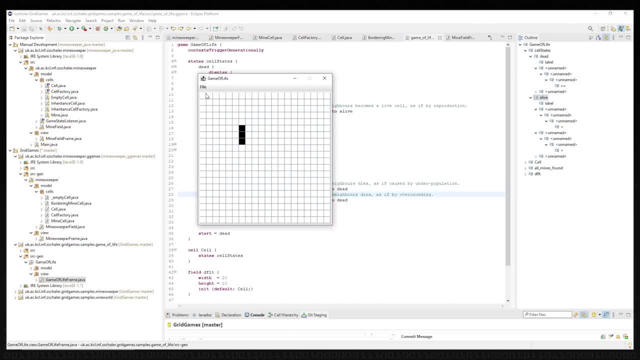 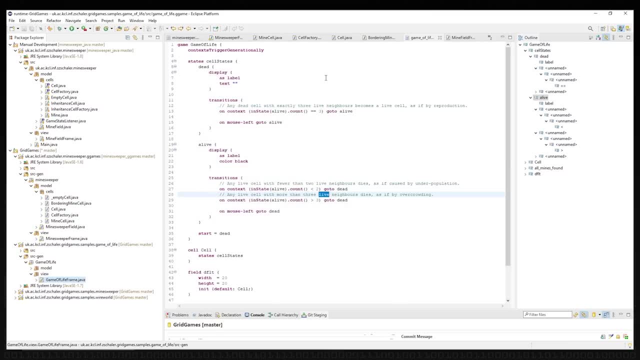 finding that kind of balance is a tricky thing, And so one other thing you can, for example, define with this language is this game of life. here We're going to scale up, I mean, you know, obviously for a simple cell program like this: 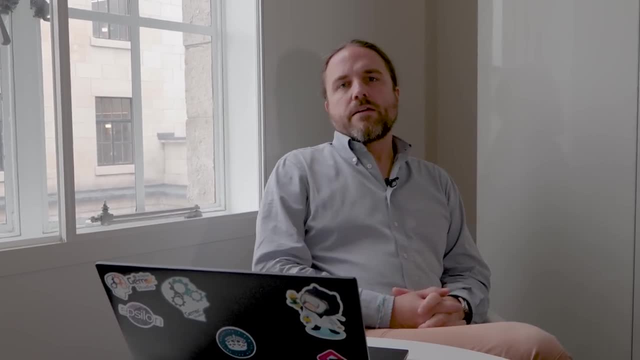 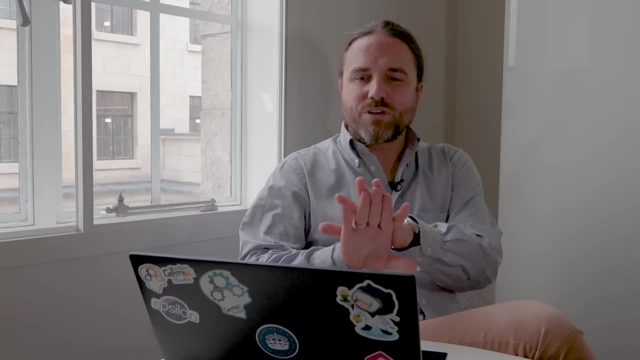 you can see this working, but we've got programs out there with millions of lines of code, haven't we? I mean, how? how would it change? No, actually, actually it scales up really well. right, Because? because what it does is. 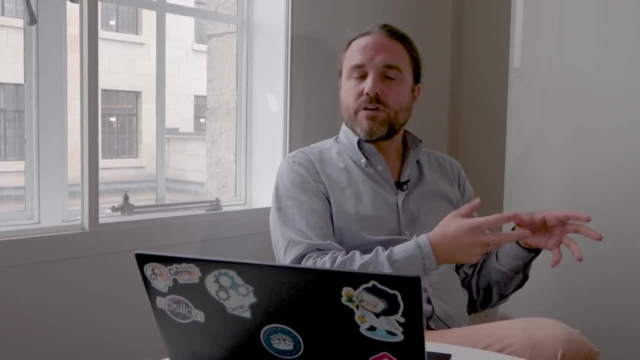 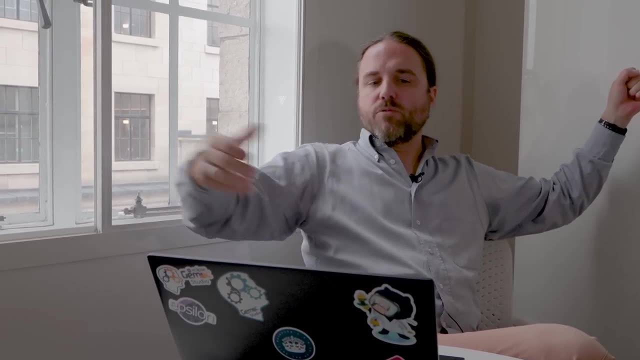 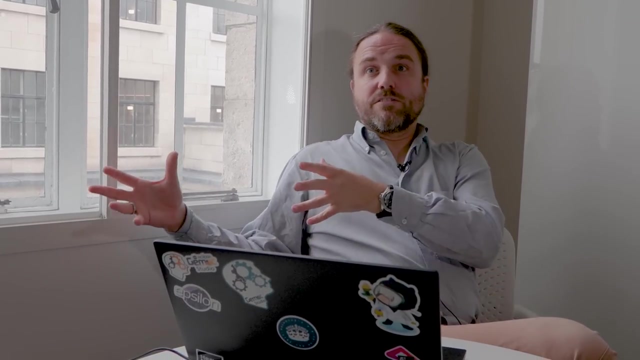 effectively reduce the number of lines of code that you write, right. So every line of code I've written here in my modeling language translates into N lines of code. I've not quite that many perhaps in this example, but potentially quite a few lines of code in in in the real sort of 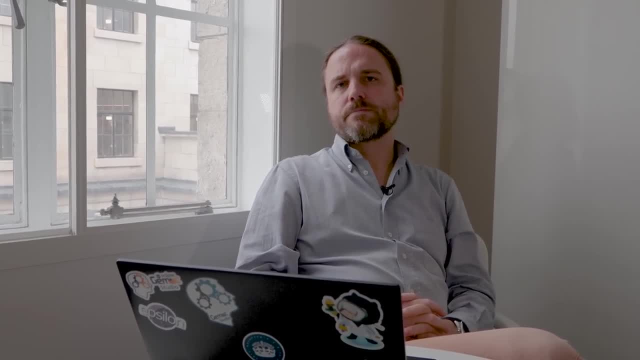 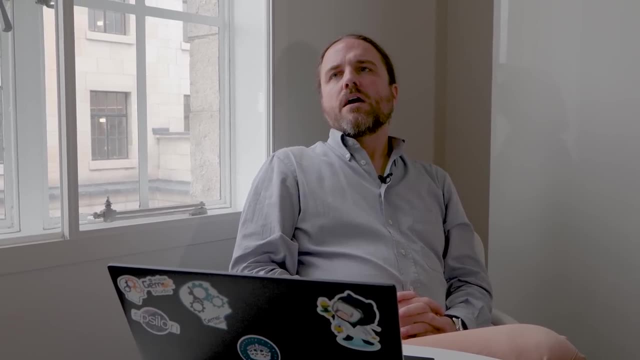 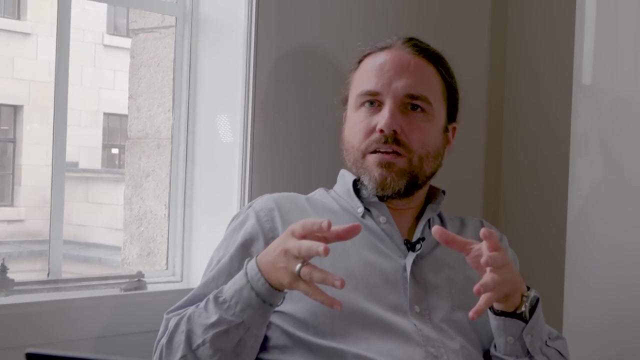 programming language. But are you not making it so it's less, less flexible process by by, you know, having to write a language for each one and then, obviously, constraining people within the what that language can do? Yes, of course, of course, Right, So you are reducing flexibility, But that's, that's always. 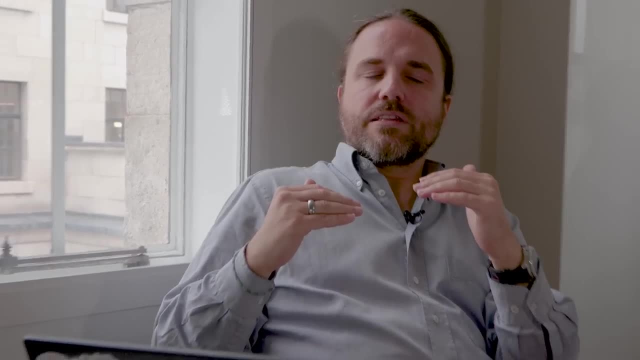 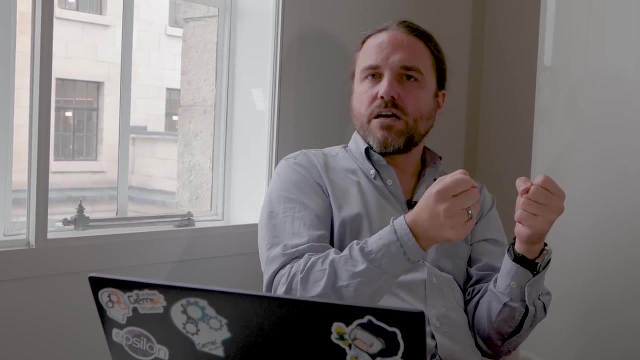 been true right In this process. So so there are things you can write in assembler that are difficult or impossible to write in a higher level programming language, but that's not necessarily a bad thing, right? Because more often than not, 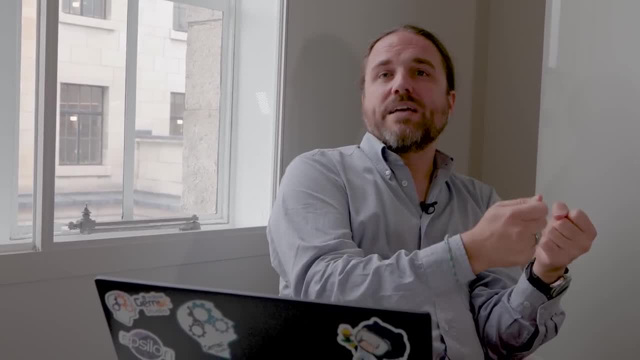 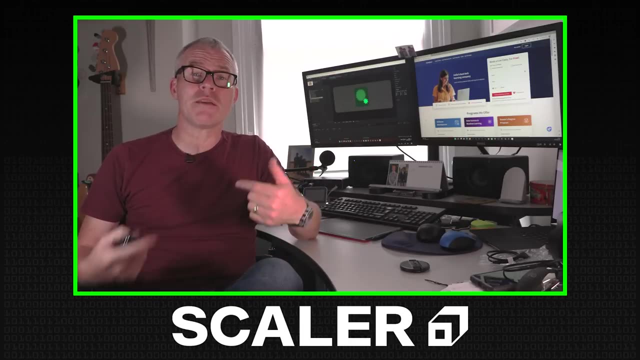 what it actually does is reduce the number of ways in which you can shoot yourself in the foot. We'd like to thank Scala for supporting this Computerphile video. If you, like me, love to learn something new, then you're going to love Scala As a resource for upskilling. 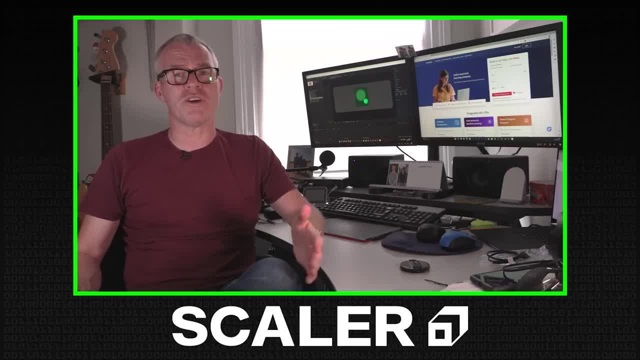 they cater to everyone, no matter what skill level, which means that you're going to get a lot out of their programs, Whether it's their interview hacks, the mentorships or curated computer science courses. every techie should know about Scala. Scala's programs are: